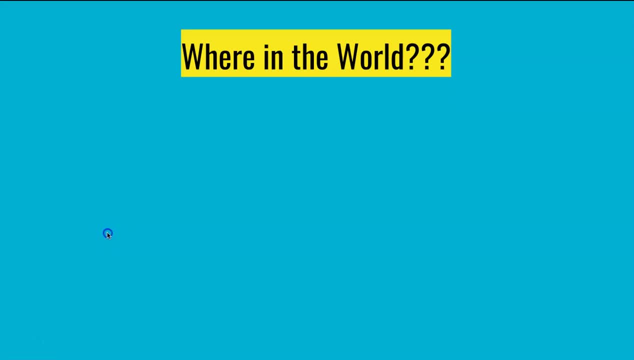 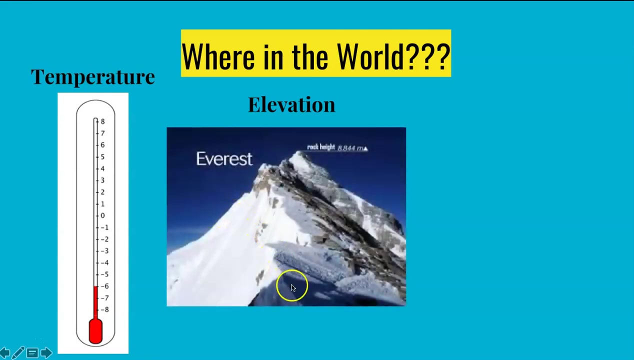 Where in the real world do we see negative numbers? An example that's often used on the EOG is temperature, because temperature includes negative numbers and positive numbers. Also often on the EOG you see elevation. We can talk about Mount Everest or another mountain and its distance above sea level. Mount Everest is 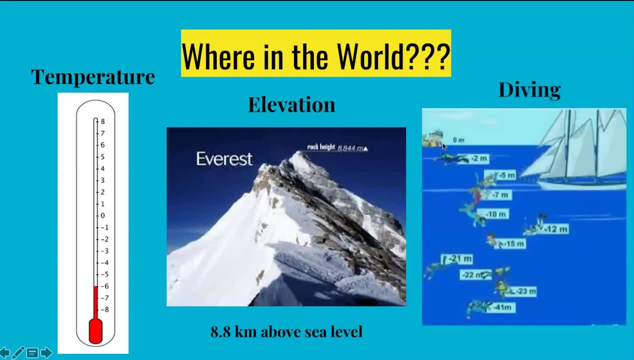 8.8 kilometers above sea level. We could also talk about locations below sea level. Here's sea level, Right here, where the water meets the sky. it's the average level of the sea. This diver is 2 meters below sea level, so it's a negative 2.. This diver is 10 meters. 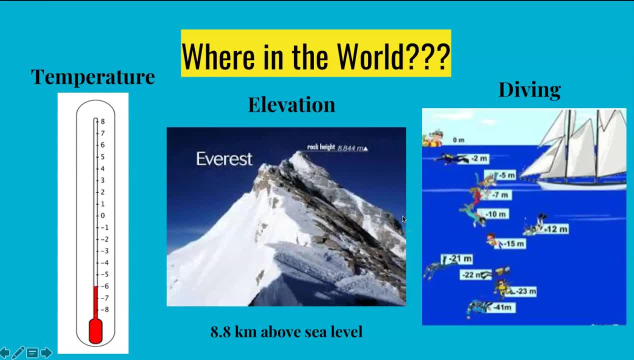 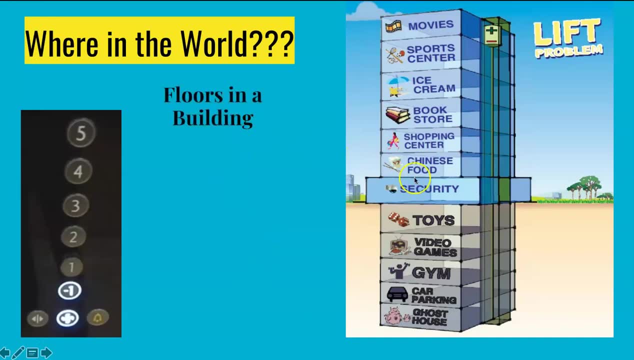 below sea level, so that says a negative 10.. I think you get the idea. Here's another example that I see a lot of times When you have floors in a building that they talk about In this example. in the United States we normally call 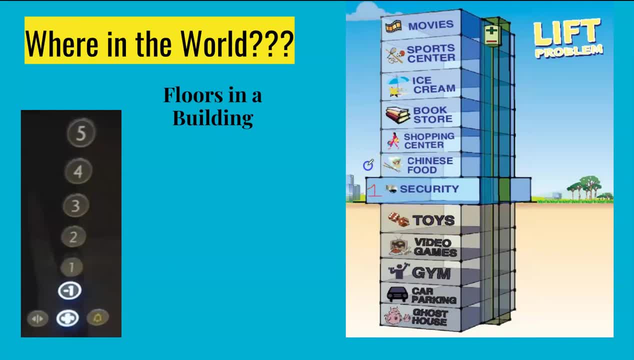 this floor, floor one, and then floor two, floor three. I really honestly prefer how they do it in Europe and some other countries. when we're talking about integers, For example in Italy, they would call the first floor. that is above ground. they would call that floor. 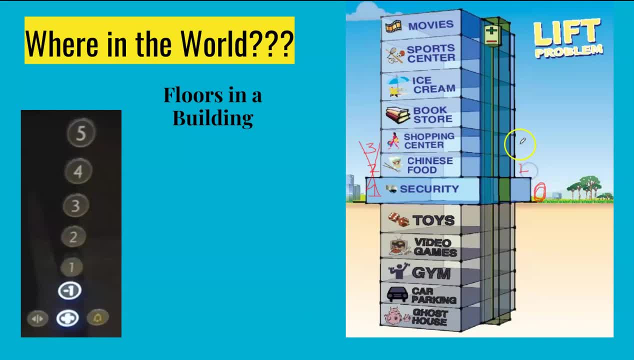 zero, Then this would be floor one, this would be floor two, this would be floor three. Okay, you get that. Then it makes it so that the levels below ground are negative numbers, So negative one, negative two, negative three. I thought this was a pretty interesting example. 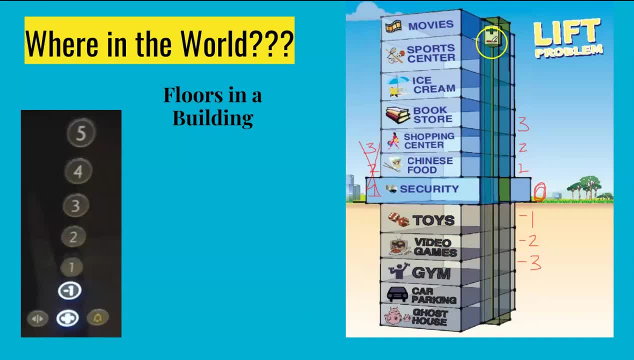 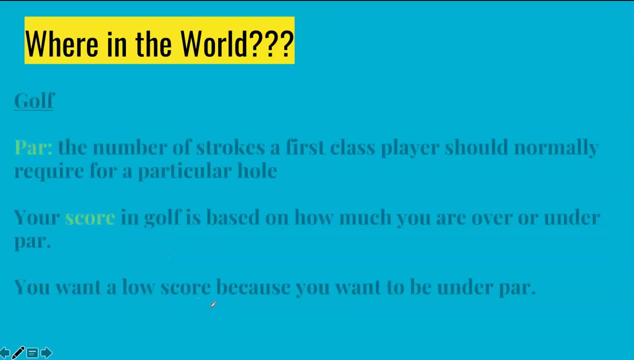 The elevator example, where as you move upwards that's positive and as the elevator moves downwards that's negative. I pulled this picture that someone took of an elevator and look there's a negative one. I thought that was interesting. Another example that we talk about often with integers is golf. I want to make sure. 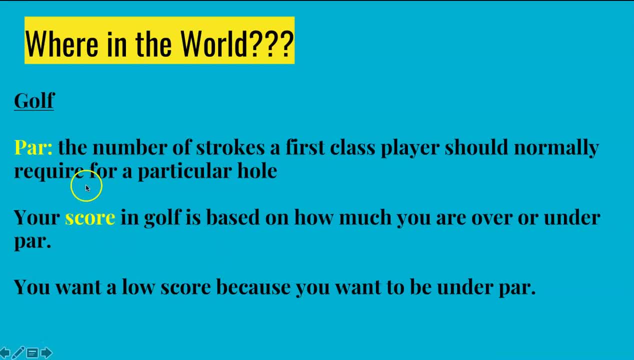 you understand this, because a lot of times kids don't understand this. Par is the number of strokes a first class player should normally require for a particular hole. You might already know this because we live close to Pinehurst and that's like golf mecca, where there's a ton of